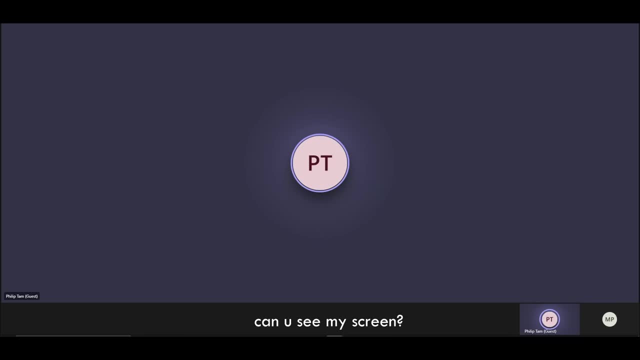 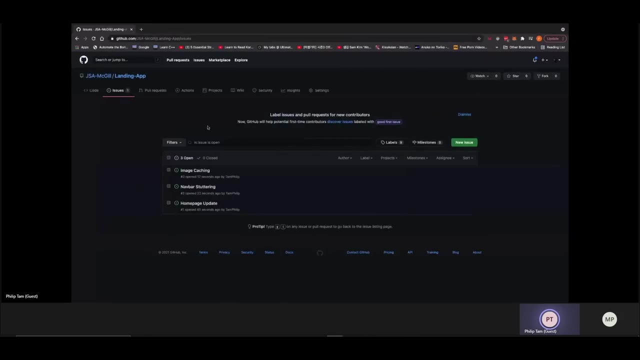 So go ahead and clone the git repository. Can you see my screen? Yeah, now I see it. Easy, I know how to do this. All right, So now you want to go ahead and install npm, node, git vs code, or you can use any IDE you want. Then you want to use your email to sign. 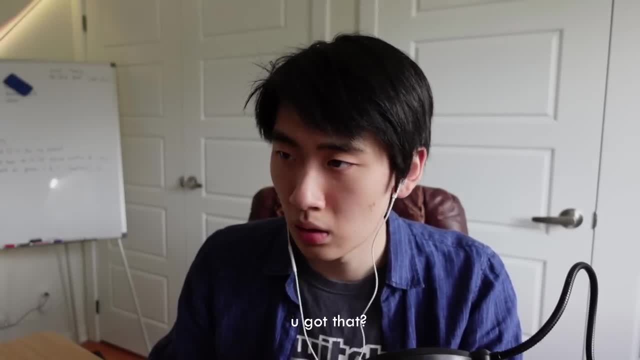 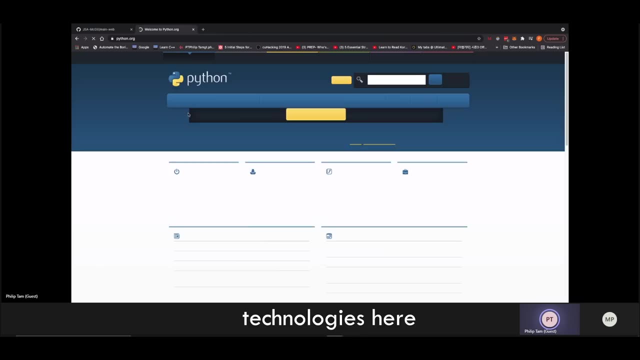 into Confluence for documentation, Azure, DevOps, Jira and GitHub. You got that, Yeah, it's just downloading. Yeah, perfect. So we're a pretty diverse company. We use a lot of different technologies here, So you want to go ahead and also install Python, Java, C-hashtag, C++. 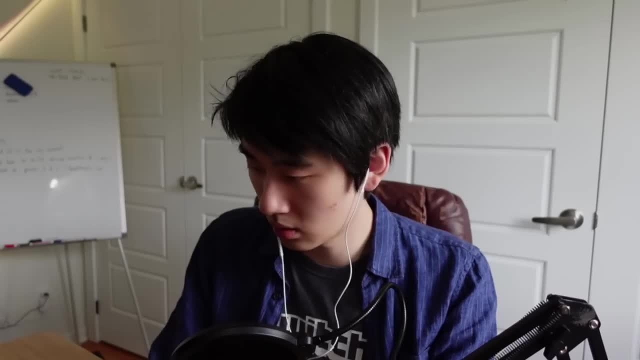 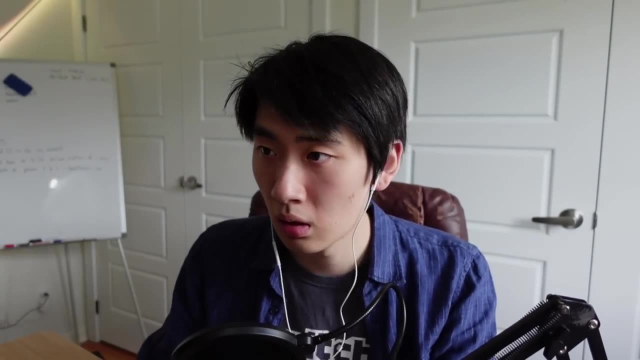 and once you get that code base set up, you want to go ahead and use the command line to directly install Linux TypeScript JavaScript and set up the configurations. I won't show you that because you know it's just. you know it's pretty simple. So yeah, do you have any questions? 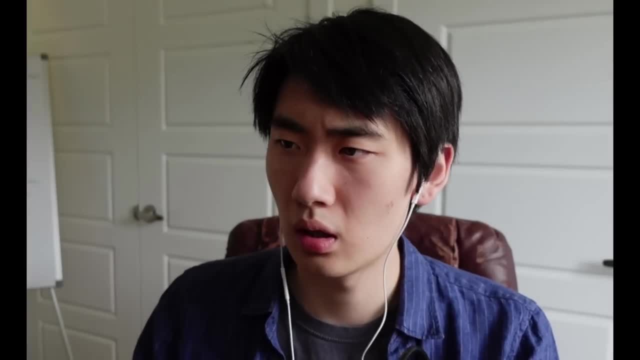 Yeah, I think your screen is lagging, All right, so, no questions. Perfect, You seem to be pretty bright. I'll give you your first task right away. It's pretty basic, you know, just to get your feedback. So I'm going to go ahead and install the code base. So I'm going to go ahead and install. 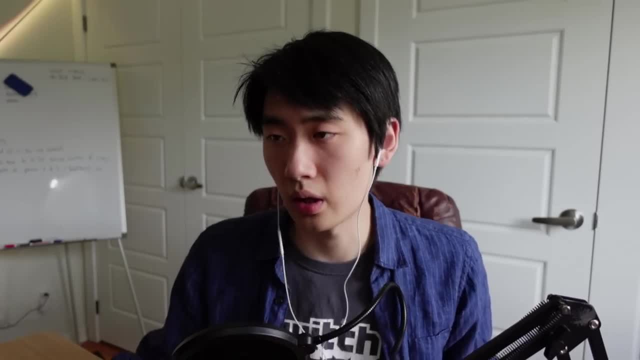 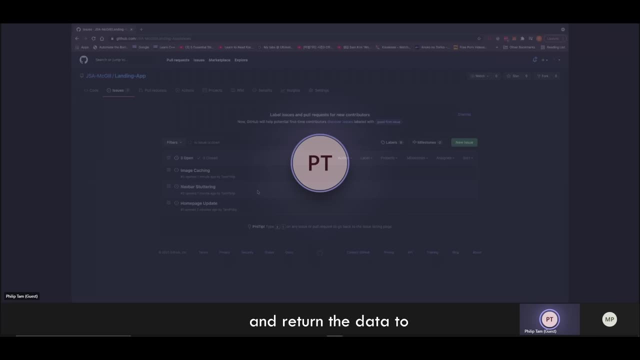 So basically, you're going to fix this button- Oh, okay, that's not too bad. And then you want to make this button interact from front to back end. it should make exactly 7.5 API calls and return the data to the AWS Cloud, WordPress, which is our middle end. But you want to make sure it. 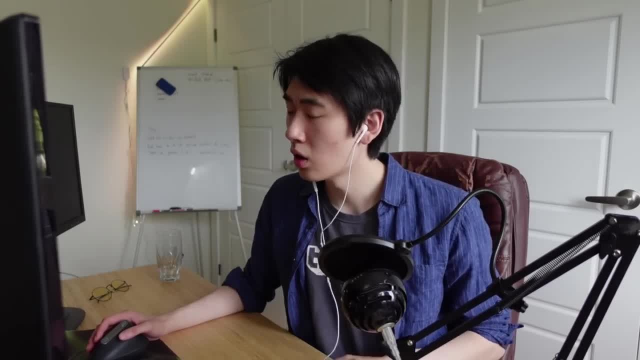 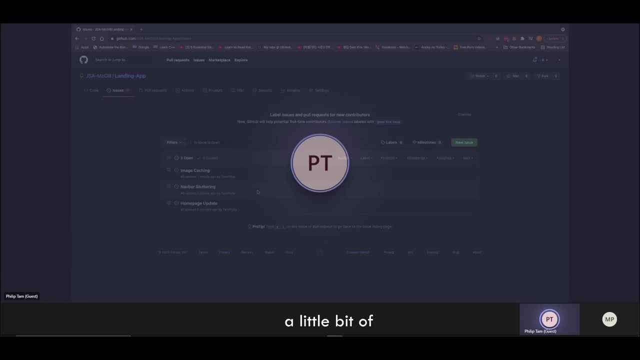 doesn't bottleneck. So add some multi threading in the JavaScript. And are you familiar with machine learning? No, Yeah, you probably are right. You kids are really good with that stuff nowadays. So maybe just add a little bit of unsupervised classification And we can, you know. 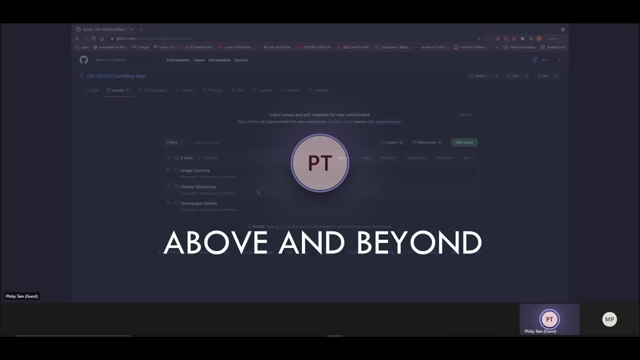 cluster the HTML attributes, And if you really want to go above and beyond, you can also use bootstrap to strap everything together at the end. You know, just pretty simple. I have to jump in on another call, So don't hesitate to ask me if you have any questions, And you'll be done with this. in like one hour, right? So I'll see you then. Good luck.